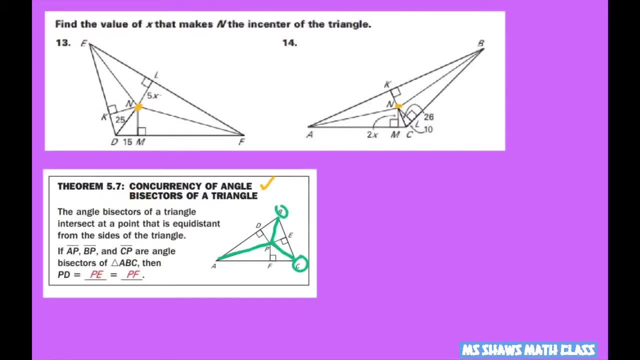 so bisecting B, C and A, and they intersect at a point that is equal distance from the sides, So these would be right angles here. So let's get started with the first one, And we're going to be using Pythagorean triples. 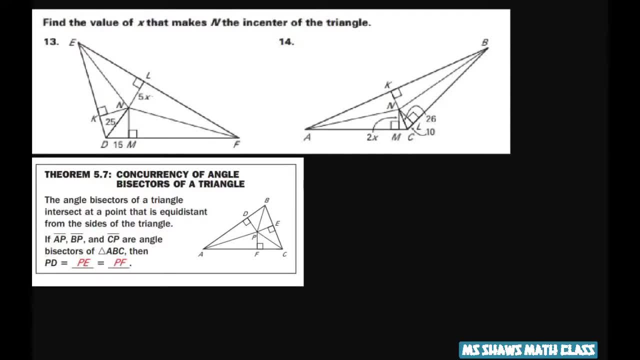 So in geometry a lot of times they use Pythagorean triples. So you're going to be using Pythagorean triples. So you're going to be using Pythagorean triples. So you don't have to always use the Pythagorean theorem if you know your triples. 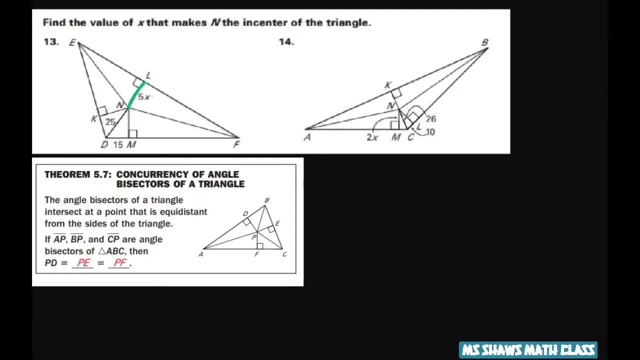 So we need to find x here, And I have this triangle here. I know that these are my angle bisectors, So I also know that these sides are congruent. So what I'm going to do is I'm going to use the triangle here. 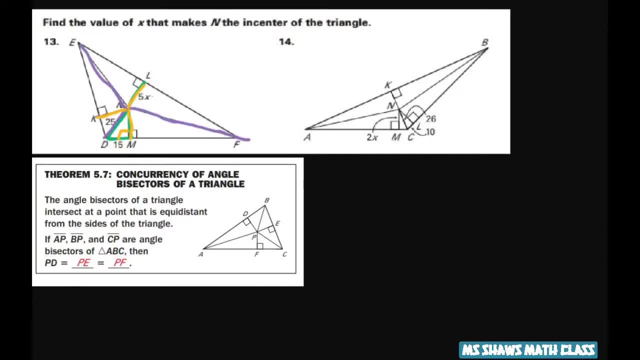 So what I'm going to do is look at this triangle right here And I have 15 and I have 25.. Now, if I divide these by 3,, I get 5.. And or by 3, let's divide by 5,, sorry. 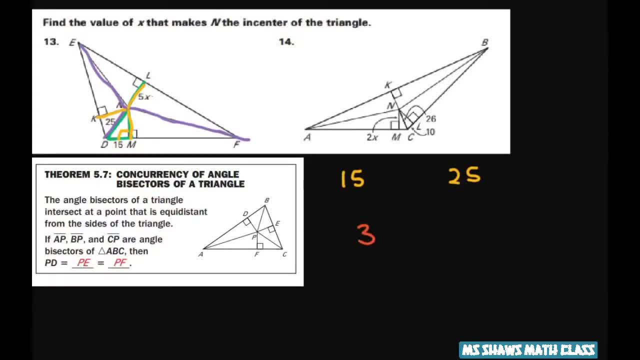 If you divide by 5, you're going to get 3 and 5.. And that should tell you that this is a Pythagorean triple. So 3,, 4, 5 is a Pythagorean triple. If you multiply this by 5, you're going to get 15,, 20, and then 25.. 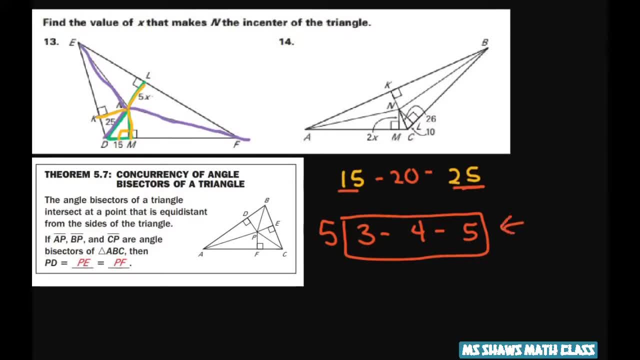 So we didn't use the Pythagorean theorem because we knew our triples. And then this side has to be 20, so this side has to be 20.. So what we're going to do is take 5x, equals has to be 20.. 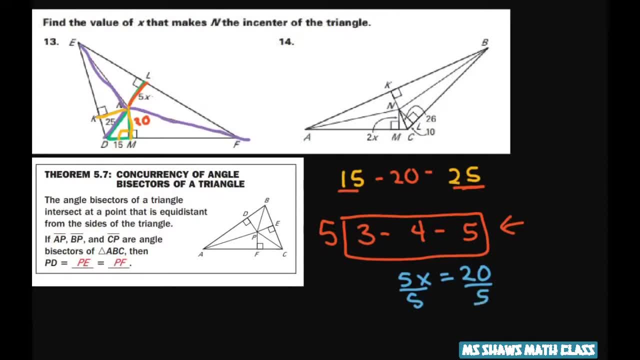 Therefore, if you divide both sides by 5, x equals 4.. All right, and we're going to do the same thing with the next one. Here's your angle, bisectors. It's bisecting A, B and C.